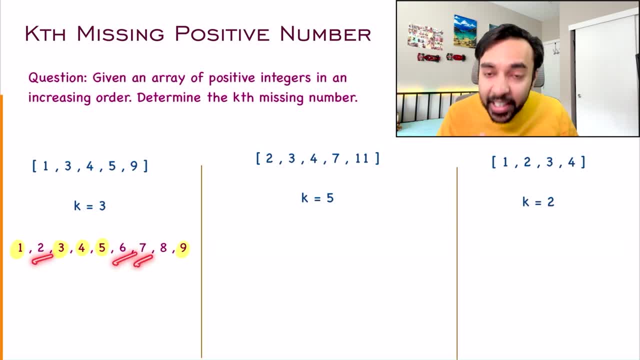 missing. 2 is missing, 6 is missing, 7 is missing and 8 is missing. The problem asks you that. okay, tell me the third missing number. So which is the third missing number? 2 is missing, 6 is. 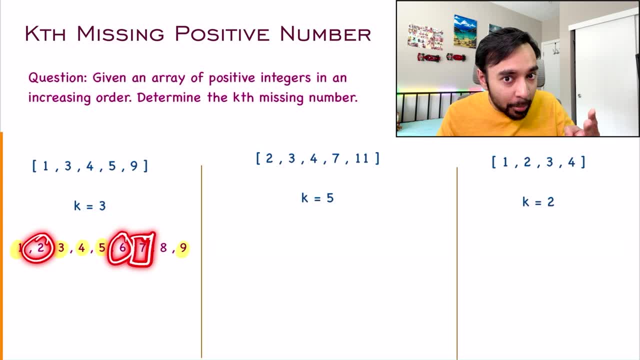 missing. and then 7 is missing. 7 is the third number, correct. So for this particular test case, 7 will be your answer, right. Similarly, when you look at your second test case, this time your array starts from the number 2,, correct, And the value of k is 5.. So, once again, 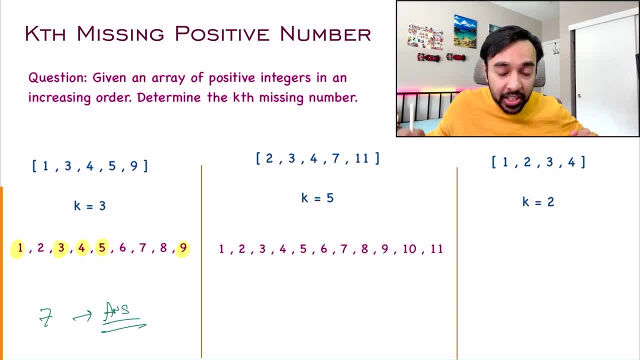 what do you do? Just start writing down all the positive integers. And which numbers have I already covered? I have a 2 over here, I have a 3,, I have a 4.. I have a 7, and I have an 11, correct? So what are my missing numbers? 1 is the first missing. 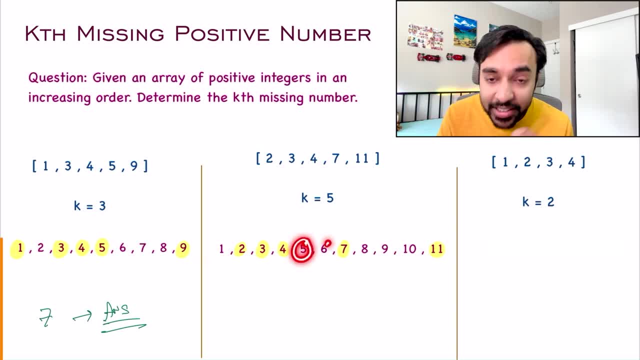 number 5 is the second missing number, 6 is the third missing number, 8 is the fourth missing number and 9 is the fifth missing number. The value of k is 5.. So for this particular test case, 9 is your answer right. So this is a scenario when you can find the missing number within the 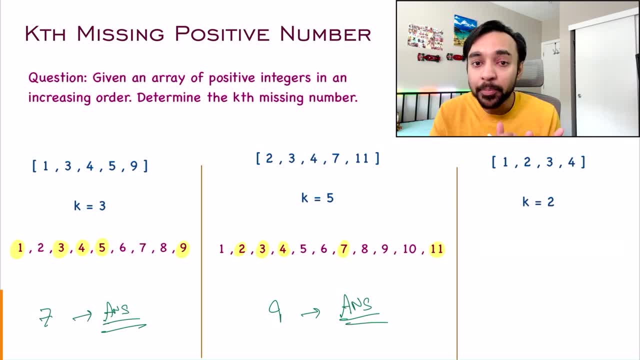 range of your array. The last test case. it's kind of tricky. You have an array 1,, 2,, 3,, 4.. And then I'm asking you: okay, tell me the second missing number. You would say that, okay, I'm starting from the beginning, and 1,, 2,, 3,, 4,. 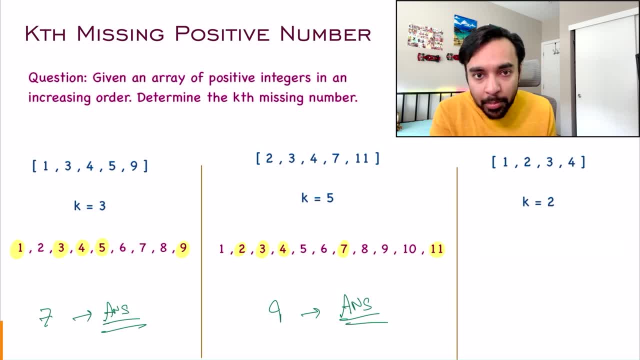 all the numbers are occupied, correct. But instead follow the same approach: Write down all of the integers. When you start writing them down now, check what numbers have you already covered. You have covered 1,, 2,, 3, and then a 4, right? I am asking you, tell me the second missing. 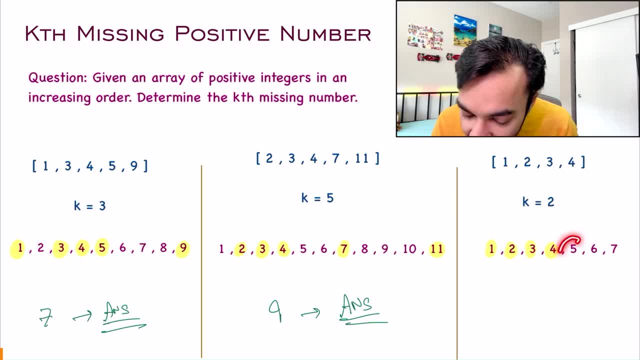 number, The value of k is 2.. So the first missing number is 5, and the second missing number is 6.. So for this particular test, case, 6 will be your answer. So this is what, particularly, you have to do in the question. If you feel that now you have understood it even better, feel free to first try. 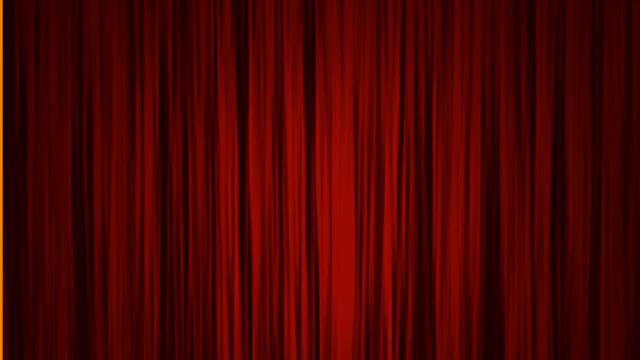 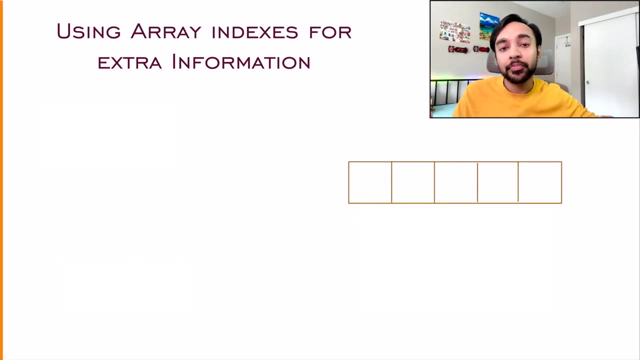 it out. Otherwise, let us dive into the solution. To come up with a solution, we must first understand what all information can we derive from an array data structure. So right now my array is full correct. An array gives you two pieces of information. The first piece of information are: 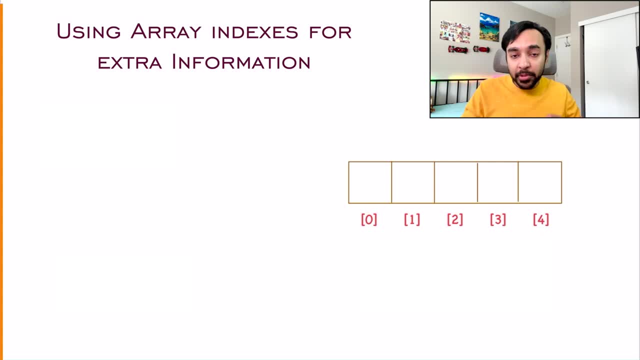 all the numbers themselves, And the second piece of information that you get are all of the array indexes, right? Why are these indexes important? Let us say I have a condition where none of the numbers are missing, So my array will be something like this: So this is the condition when none of 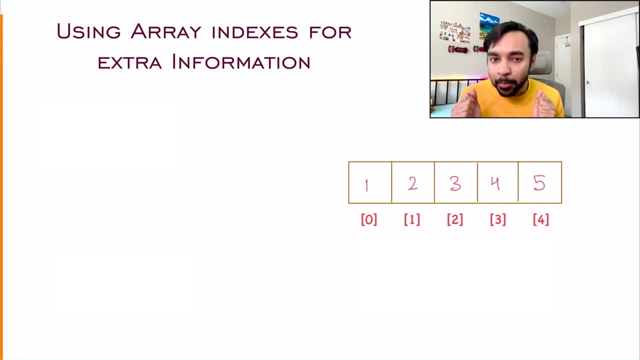 the numbers are missing, right? And how can you derive these numbers closely? each of these numbers are one greater than the index, right? So if your array is very huge, let us say you have a hundred elements, then at the hundredth position, if no number was, 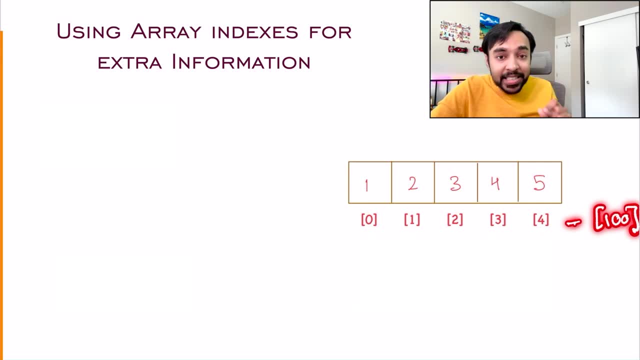 missing, what will be the number over here? That will be this index plus one. that means one, zero one. So these indices, they can determine that, if no number was missing, what should be the element at this particular position? right, So we can derive all of these numbers just by adding a. 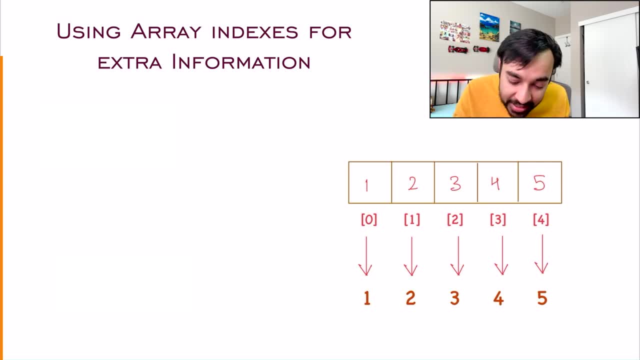 one. So if we see any discrepancy in any of these elements, we should be able to identify it correct. So that is the technique we are going to use. We already know that at these positions, this should be the number when none of the numbers are missing right But over here. 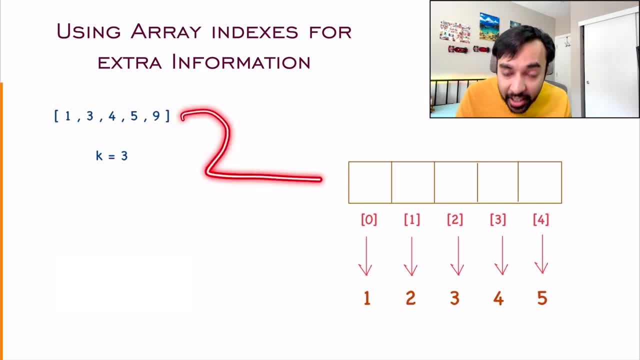 I have the sample test case and we will try to plug in all of the values. Remember that you have to find out the third missing number. but we will get over there, Just stay with me and it will become perfectly clear. So I will try to populate in the first number. I get a one And if you notice, 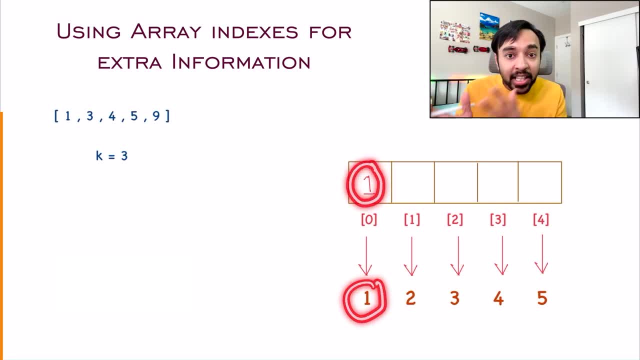 the element should have been a one over here. That means none of the numbers are missing up till this point. And you can also find it out by one minus one, And that gives you a zero. That means, up till this point, zero numbers are missing. No numbers are missing at this point. correct Populate: the next value. 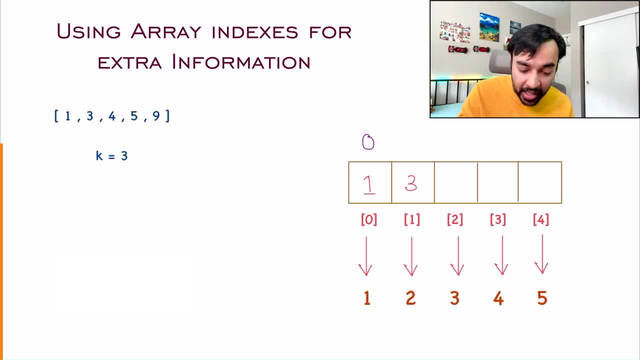 now, The next value you have over here is three And if you notice, this index is telling me that the value over here should have been a two instead, right? So that means some numbers are missing. How many numbers are missing? You find it out by three minus two. So three minus two: 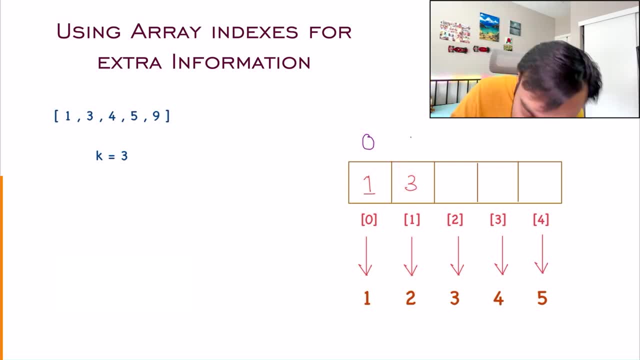 and that gives you one. So I know that Up till this point, one number is missing, correct? That number is in fact two. right, You have to find out the third missing number. So you can be very sure that, up till this point, 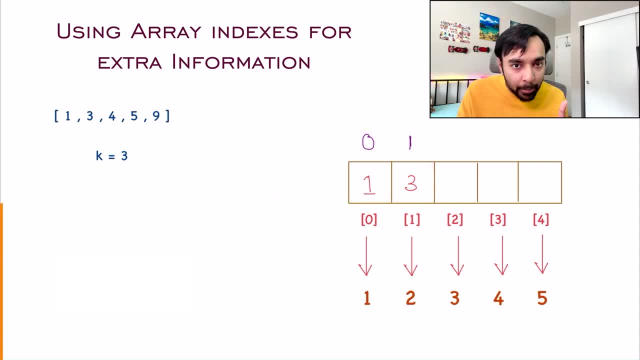 you won't find it, Because up till now, only one number is missing. Now move ahead. The next number you have is four, But instead you should have a three over here, correct? So once again, what do you do? Four minus three, and that gives you one again. Up to this point. 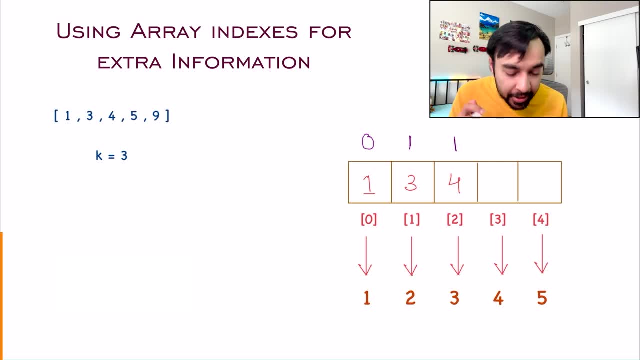 also. only one number is missing, So we can keep going ahead. The next number is five And according to the array index, four should have been over here. So to find out how many numbers are missing, you do five minus four, and that gives you a one again. So up till this point I know that only. 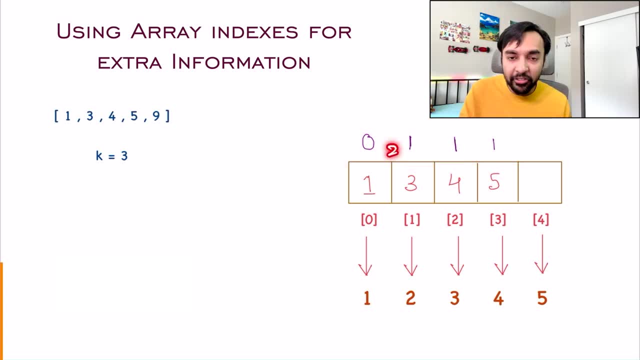 one number is missing in my array. That was the number two. in fact, right Now, populate the last number and things will get clear. The last number I populate is nine, But according to this index, five should have been at this place, And that is telling me that some 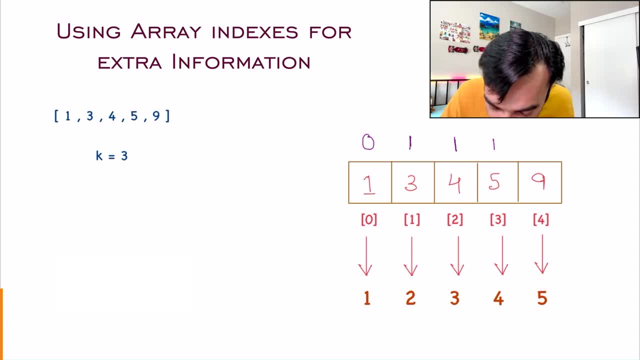 more numbers have gone missing, And how many numbers are missing. Nine minus five, and that gives you four. So up till this location, four numbers have gone missing. Now I have a very important piece of information available At every location, I know how many numbers have gone. 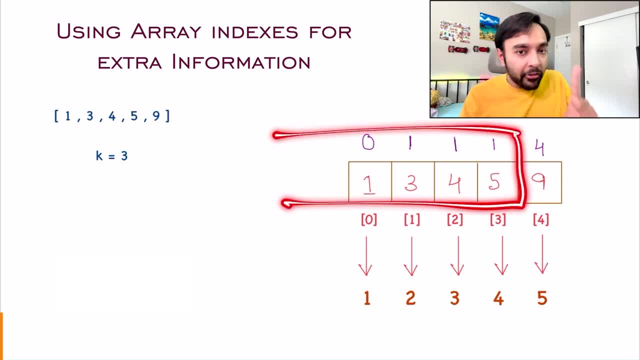 missing. So up till this location, only one number was missing. So up till now, only one number was was missing right. And suddenly, at the last location, four numbers have gone missing. You have to find out the third missing number, right. So definitely this third missing number that will. 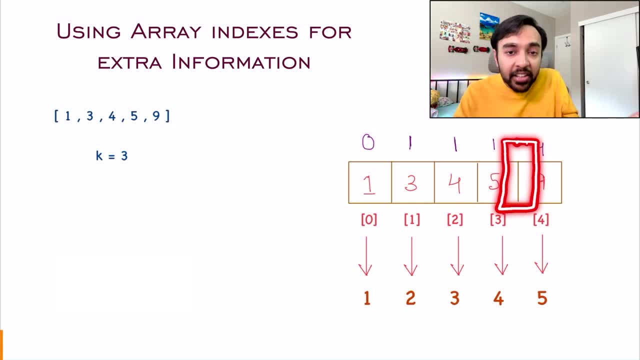 be somewhere between here. That means between 5 and 9,, correct? And you already know that up till 5, only one number was missing, right? You have to tell me the third missing number, So I can do 3 minus 1 and that is a 2,, correct? That means after 5,. if I find out two more numbers, that 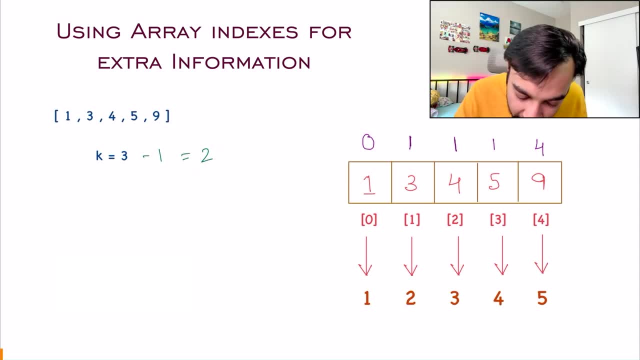 will be my answer correct. So what we do is we take 5 and then plus 2, so that gives me a 7.. And that is exactly what we did right Up till 5, you only had one missing number right, And that. 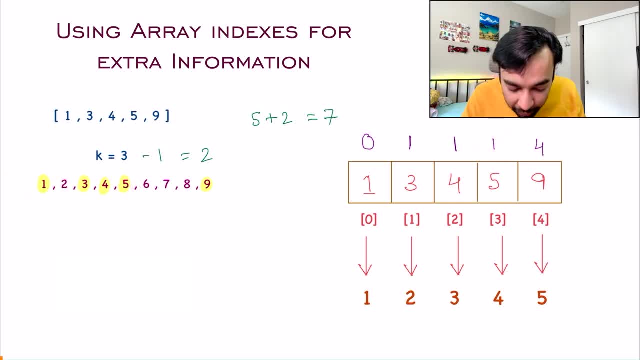 was 2.. You find it out over here and then you have to tell me the third missing number. So you do 3 minus 1 and that is a 2, correct, That means after 5,. if I find out two more numbers, that will be my. 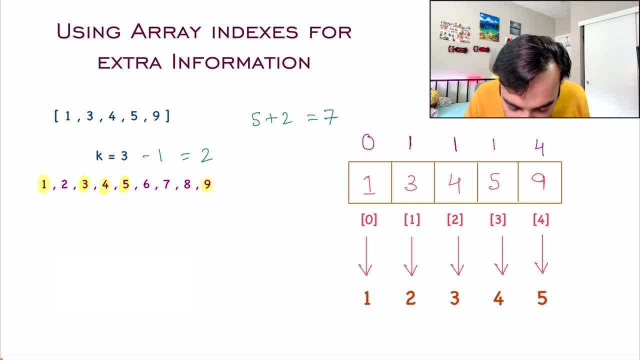 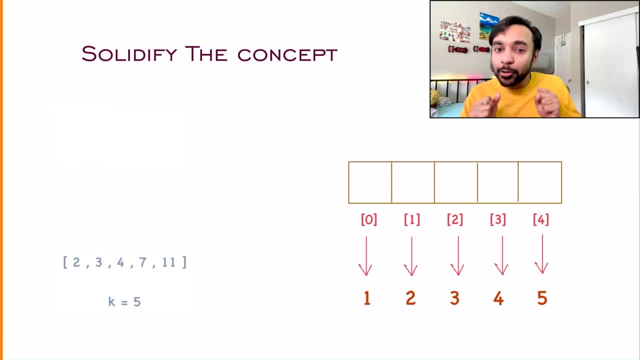 answer: 3 minus 1, and that gives you a 2.. So you move two spaces ahead and you get this number, which is your answer right. To solidify this concept, let us look at one more test case Over here. I have this array right And what I will do is I will start populating these elements. 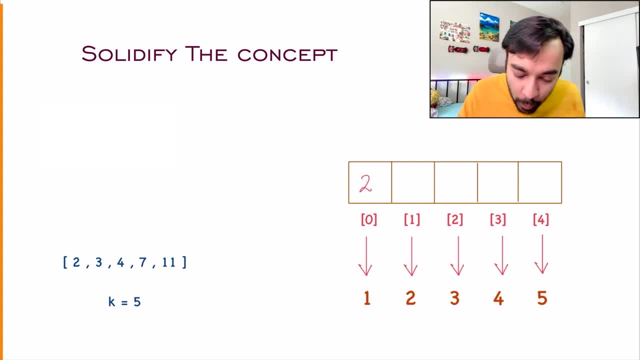 one by one. The first element I have over here is a 2. And from this index I know that the first element should have been a 1 in fact. So up till this point, how many numbers are missing? That is 2 minus 1 and it gives you a 1.. So I know that, up till the first location, only one number. 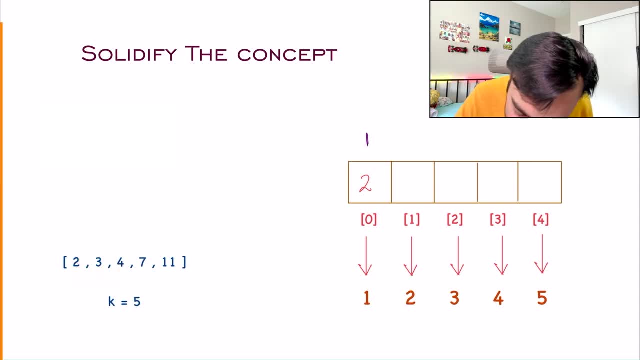 is missing. right, Populate your second element now. The second element is 3,, but according to this index, the element should have been 2.. So how many numbers are missing? 3 minus 2, and that is a 1.. Go on to the next number. You have a 4.. According to the index, it should have been a 3.. So how many? 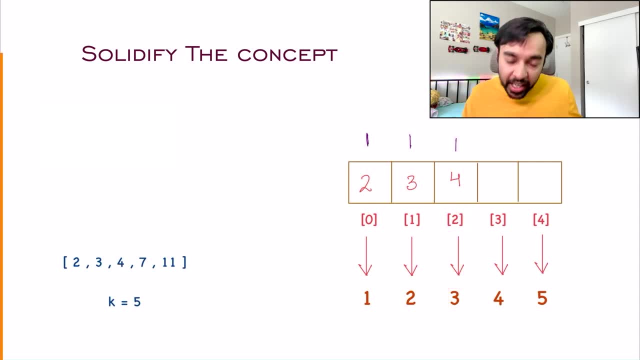 numbers are missing: 4 minus 3, and that is a 1.. Move ahead number is 7.. But according to this index, the number should have been 4 over here. So how many numbers are missing? 7 minus 4, and that gives you a 3.. So, even up till this point, only 3 numbers. 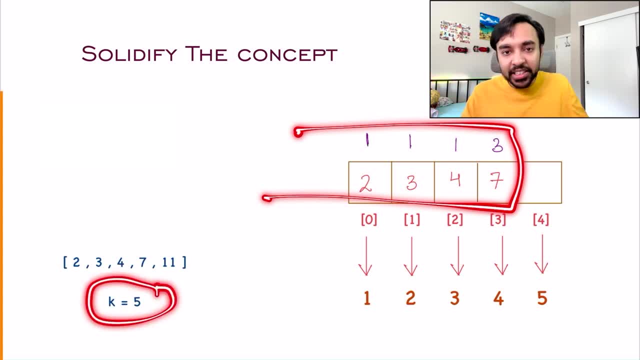 have gone missing, But I have to find out the 5th missing number. That means I have to keep moving ahead. The next number I have is 11. But according to this index it should have been a 5 over here. 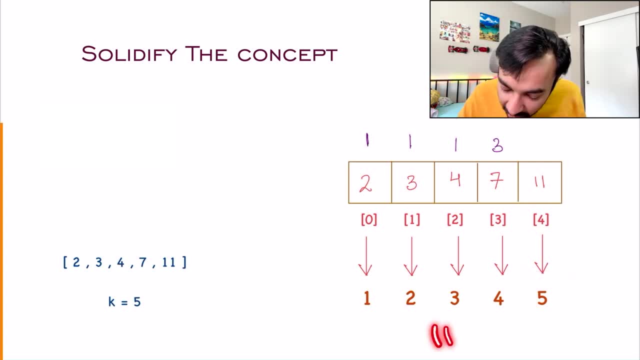 So how many numbers have gone missing? 11 minus 5, and that is a 6.. So I know that up till this location, 6 numbers have gone missing and up till this location, 3 numbers have gone missing. I have to find out the 5th missing number. So definitely I will find this 5th missing number somewhere. 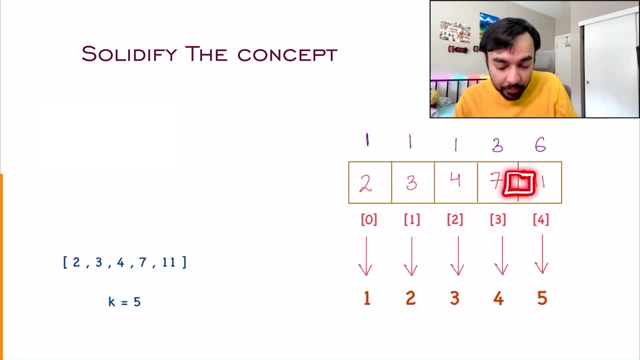 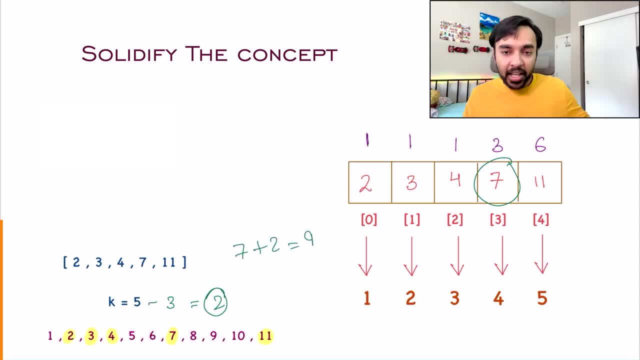 7 plus 2 and that is a 9, right. And once again, if you remember from your example, up till 2, I was missing one number and that was 1.. Up till 3, I was missing one number and that was 1.. Up till 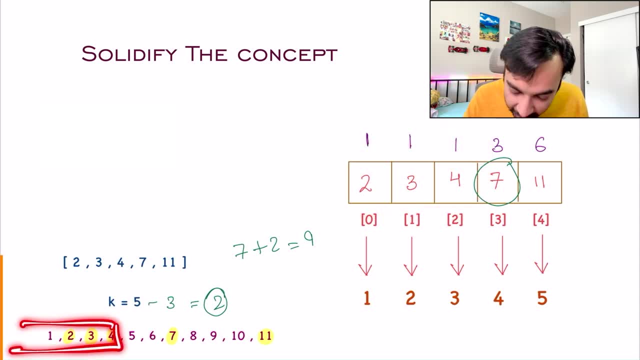 4, I was missing one number, and that was a 1. again, Up till the number 7, I am missing three numbers, and these three numbers were 1, 5 and 6.. Up till 11, I am now missing six numbers, and these are: 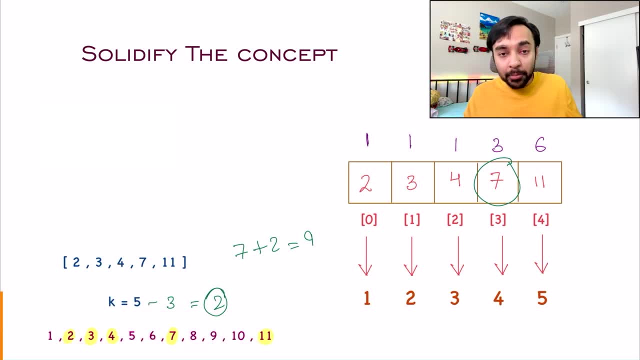 all the six numbers, You have to tell me the fifth missing number. So up till here I have missed three numbers, correct? So that is why 5 minus 3 and that gives you a 2. That means after 7,. 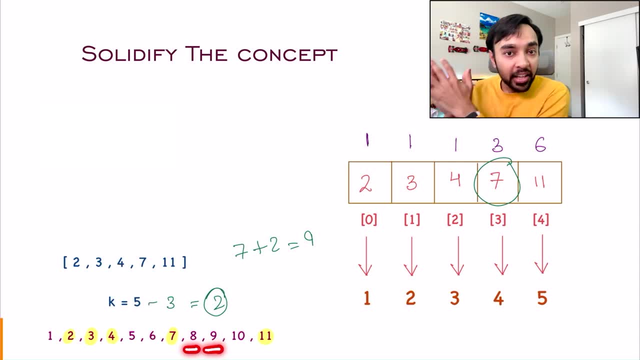 if I do 2 plus, then I will get my fifth missing number, and that is 9, which is your answer, right? So this is an approach which works in a order of n-time complexity, because you are traversing your array only once and you are just looking at all of these differences. That means just 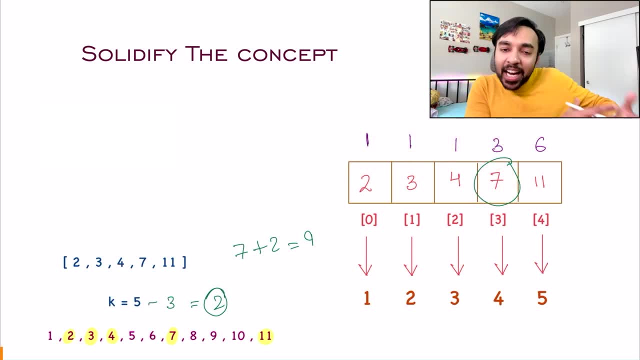 the difference of element from this index and that is telling you that, hey, these many numbers are missing. As soon as the number of missing numbers get above k, you can just apply this calculation and then find out: hey, this was the missing number. So this approach works in a 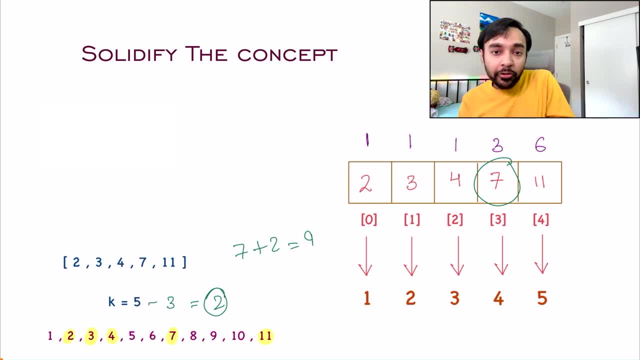 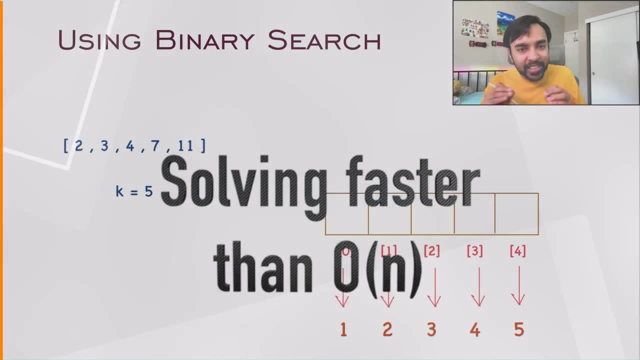 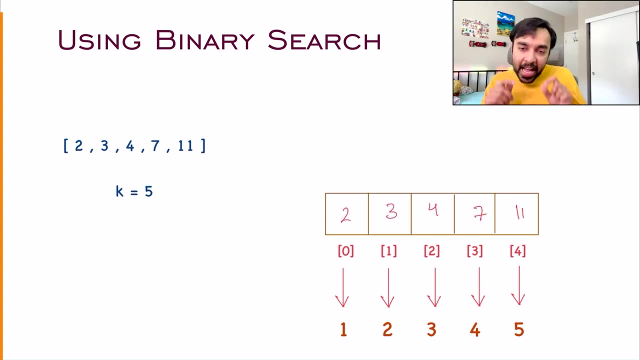 order of n-time complexity, But you have to find out a better time complexity, and that means binary search. If you have understood so far, applying the binary search algorithm is very, very simple. So, up till now, what have we done? We had all of these elements and, for every location, using these indexes, we found out how. 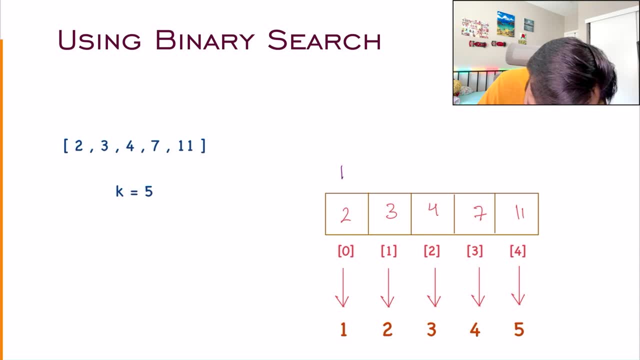 many numbers are missing, right. So 1, 1, 1, 3 and 6.. These are the missing numbers, correct. So what do you have to do? You have to find out the fifth missing number. So it becomes very, very. 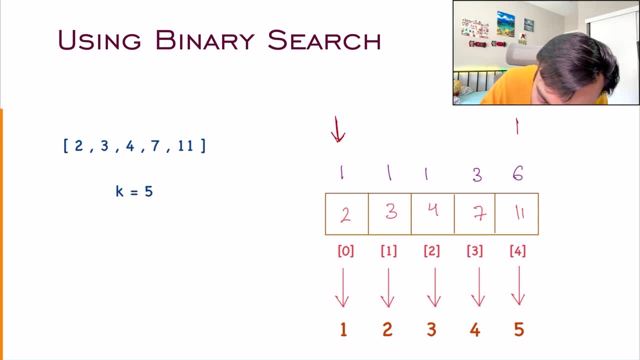 simple: You take up a low pointer and then you take up a high pointer And after that you just apply the binary search technique to find out 5 between these two indexes. Applying binary search is very, very easy. So what will happen is these pointers will start to converge in an order of log n-time. 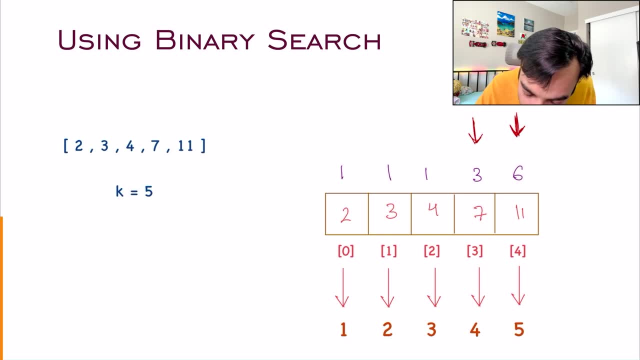 complexity And eventually you will find out that, okay, 5 will exist between these two indexes. So 5 will exist between 7 and 11, correct, You have already found out 3.. You have already found out 7.. So what do you do? You do 5 minus 3, and that gives you a 2. And then to eventually get your 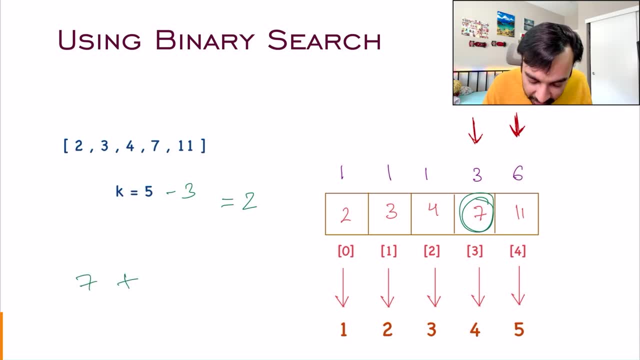 answer. you take up this element 7 and then you add up this over here And that gives you a 9.. And 9 is simply the answer. So this is how you can take the advantage of binary search to get a solution that works. in order of log n-time. 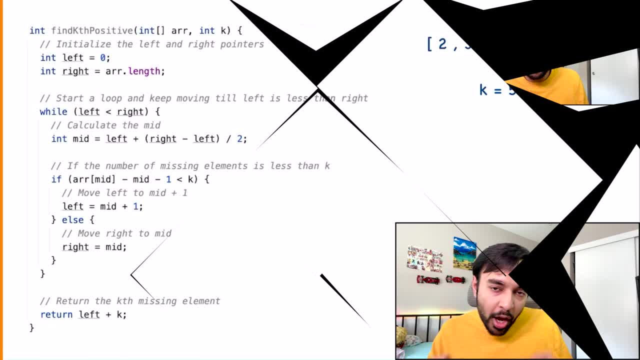 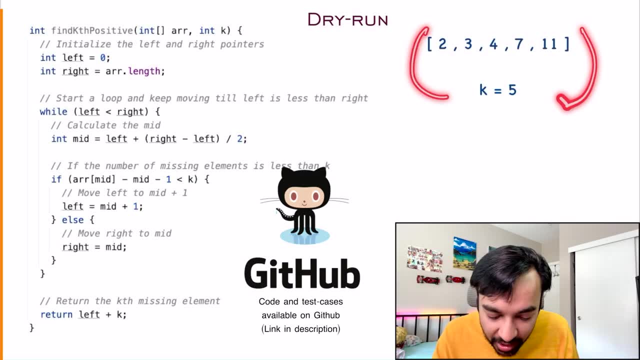 Once this is clear to you, writing the code for this is very, very simple. On the left, I have the exact code to implement this solution, And on the right I have the sample array that is passed in as an input parameter to the function findKthPositive, And notice that this code is: 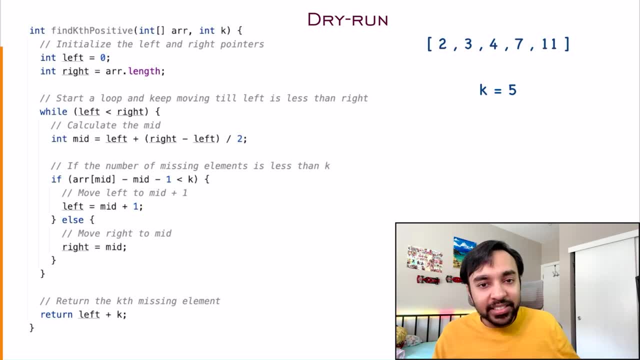 really, really simple. It is just an implementation of the binary search algorithm. You have a left pointer that starts at the first location and you have a right pointer that starts at the very last location, And then you just start a while loop until left is less than right. So, after finding the mid, 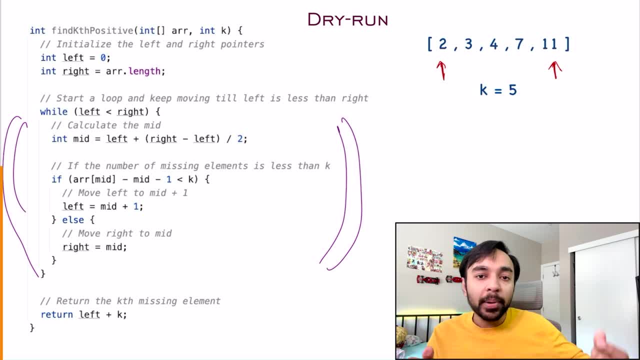 element, you will start to converge. But where do you apply the binary search? You apply the binary search on the indexes, not on the elements itself. That is why we were adding 1 to the indexes right. So just use this approach and you will be able to find out the location of the left and 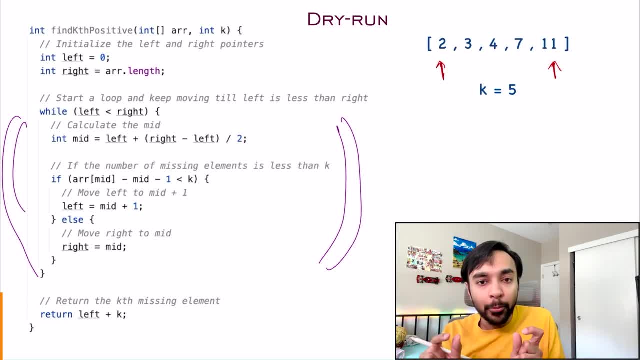 right pointers. Once you find out where the left and right pointers are returning, the element is very, very simple, right The time. complexity of this solution is order of log n, because you are performing the binary search approach, and the space complexity of this. 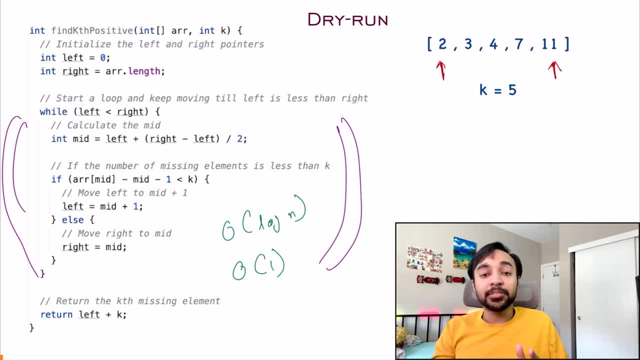 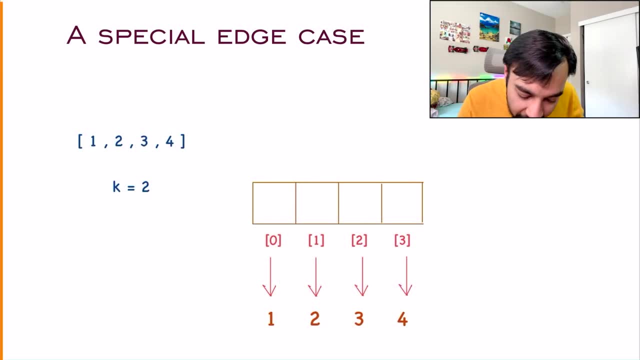 solution is order of 1, because you are not taking any extra space to arrive at your solution. I would also like to discuss one of the edge case associated with this problem. So let us say you have your sample test case like this, correct, And once you populate all 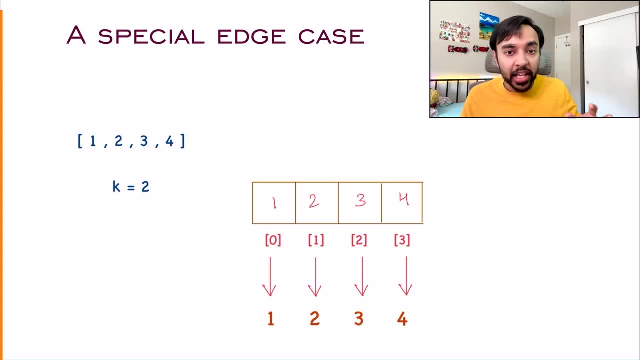 of your elements and now you try to find out: okay, how many elements do you have, How many elements are missing at every location? You will get a zero at every instance, right, Because none of the elements are missing, correct? So in such a case, if you ask me, okay, how do I find out two? 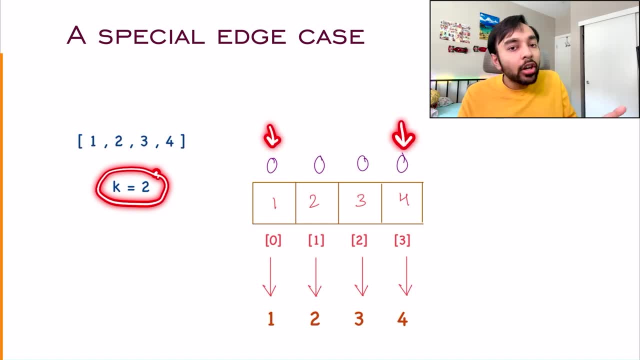 between these two locations correct When all of the elements are zero. In such a case, what will happen is when your binary search algorithm starts, both the pointers will be at the left and right location. In a binary search approach, you will look at the middle element. 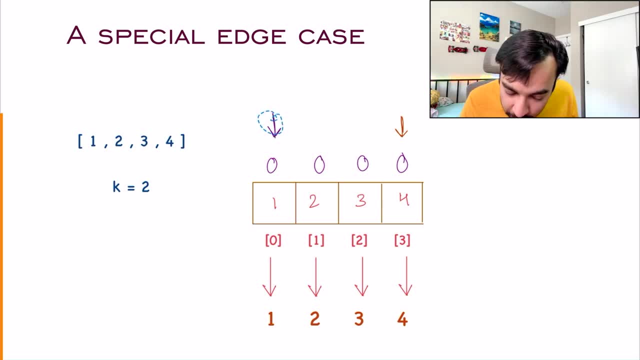 So what will binary search do? It will move the left to middle pointer And if you're not finding the element once again over here, binary search will keep on moving the left pointer. So this left and right pointer will eventually coincide and they will be at the last position itself. 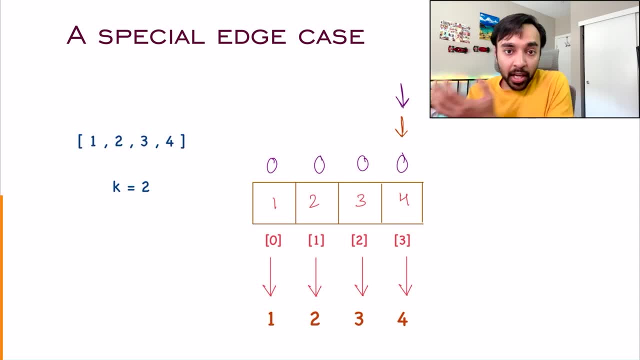 correct, And this is where you exit the loop. So you haven't found out the element and still the value of case two. So what do you do actually? You just do two minus zero. And what does that give you? Two minus zero is two again. 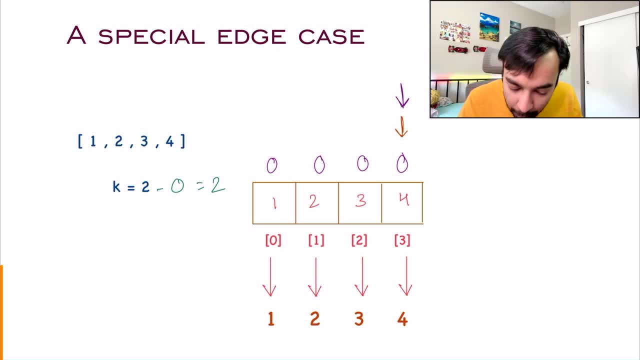 And to find out the second missing number, you once again apply the same approach. You add two to whatever element you had over here, So two plus four and that gives you a six. So once again, this gives you six, is your answer. Notice that the approach is same. 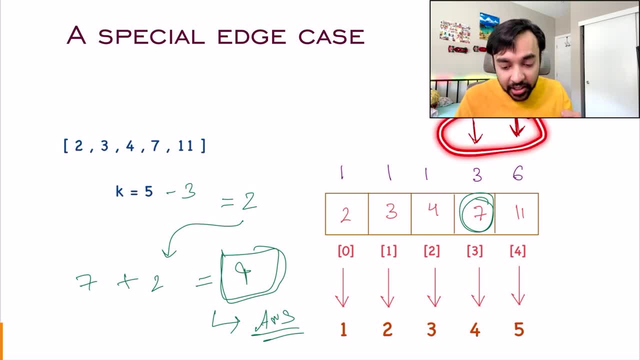 In a previous example as well. once you had the left and right pointers, the left pointer was this particular position right? So what did we do? Five minus three, and that gave us a two. And then we added this two to this element over here: Two plus seven, and that was the answer. 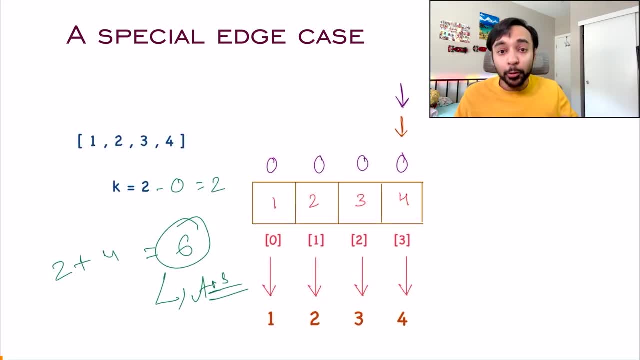 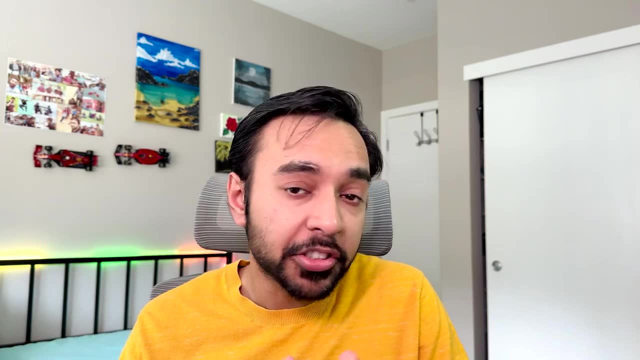 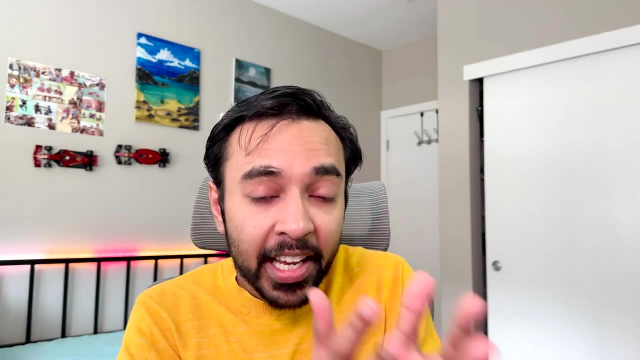 right, And this is the exact same thing that we do over here. That is why, if your concepts are clear, none of the edge cases will escape you. I hope I was able to simplify the problem and its solution for you Whenever you see a problem, or rather an interviewer asks you that hey, can you come up with. 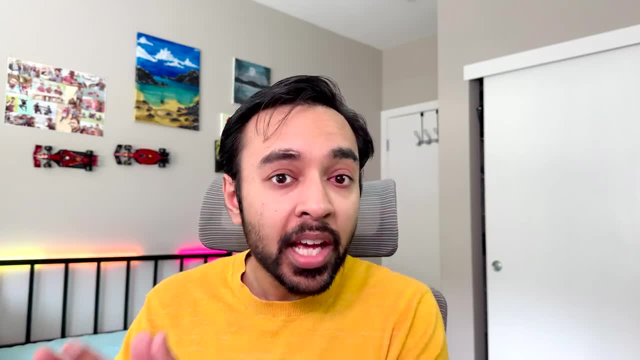 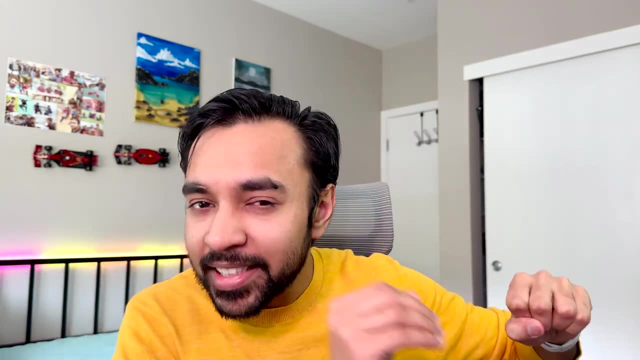 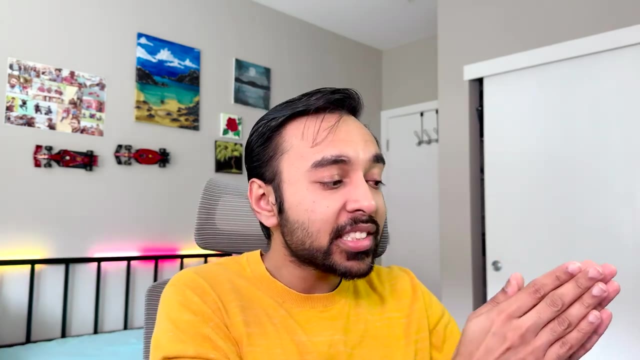 a time complexity that is better than order of n. This is a very good indicator that you have to apply the binary search technique somewhere, because that is the only way that you can reduce the time complexity less than n. A n time complexity means you are scanning every element. 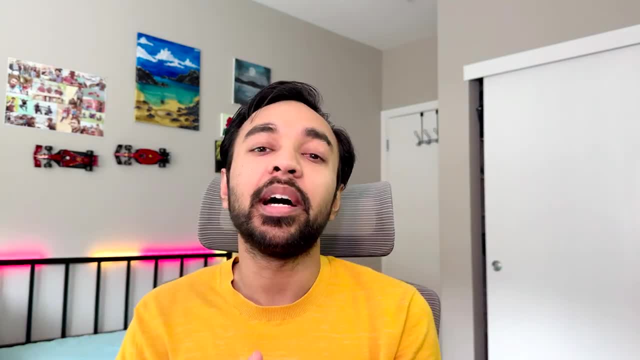 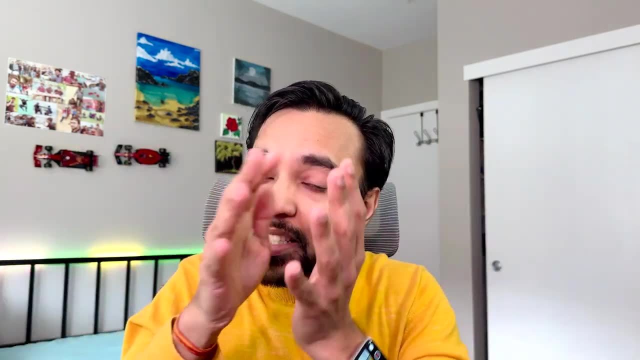 of the array, and going better than that usually means binary search. One more indicator is that whenever you have a sorted array, when things are sorted, searching can become very, very fast, thanks to the divide and conquer technique that is provided by the binary search.